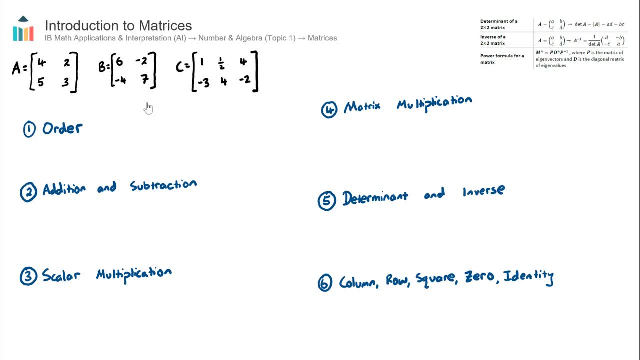 progress through some important information and concepts that you need to understand at the start of the matrix topic and then later on we'll go into more advanced concepts in future videos like solving simultaneous equations or doing long-term probability using eigenvalues and eigenvectors. But let's just cover the basics here. Let's 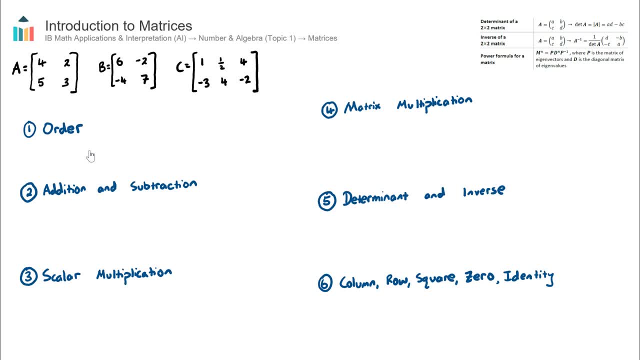 first look at the basics here. Let's first look at the basics here. Let's firstly start with how do we describe the order of a matrix, And I'll just quickly go through these three. So the order is how many rows the matrix has. So in this case, matrix A has. 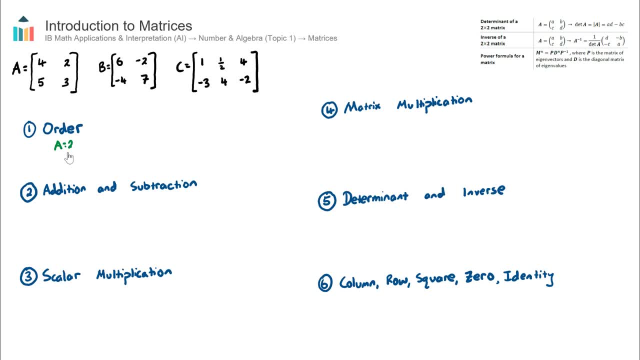 two rows multiplied by how many columns it has. So this matrix A will be a two by two. We don't actually perform the multiplication there, We just call it a two by two matrix. Likewise for B. B will also be a two by two. C, on the other hand slightly different. it still has two rows, but it has three. 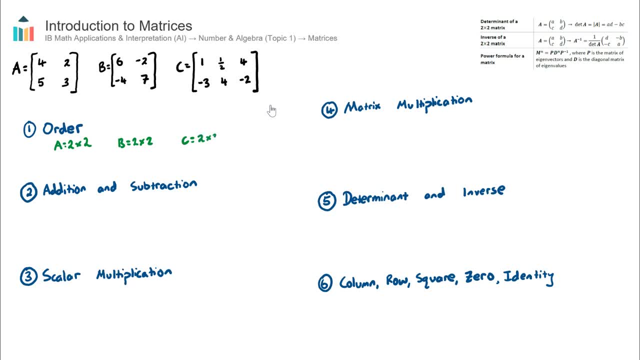 columns. So this will be a two by three. So just be careful there. in the order in which you write the numbers It's always number of rows by number of columns. Okay, let's now move on to addition and subtraction. Now you can only add or subtract matrices that have the same order. So if we look, 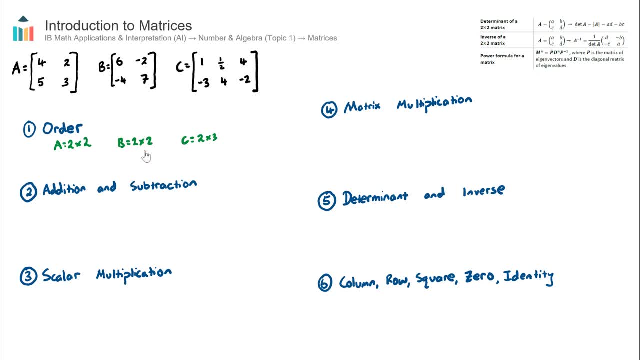 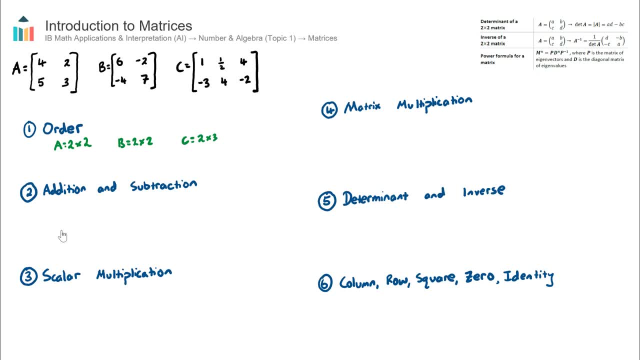 compute the addition and subtraction. So let's go ahead. I'm just going to do one example here. I'll just do addition, because subtraction is the exact same concept, just subtracting instead of adding. But let's add A plus B. Now I can add these two matrices together, because they are both. 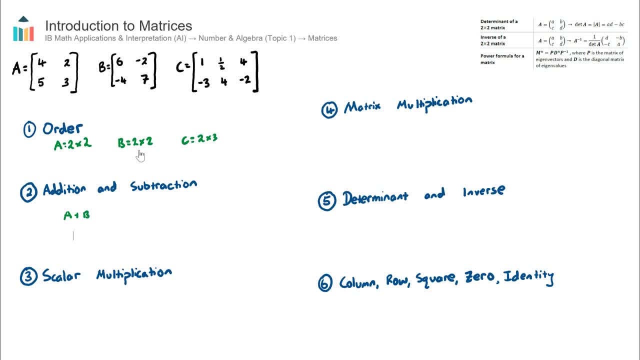 a two by two and the resultant matrix will also be a two by two. The result will also be the same order as the two that are being added or subtracted, So that will equal. I'll set up enough room here for a two by two. Now, in this top left cell or top left number, here will be: 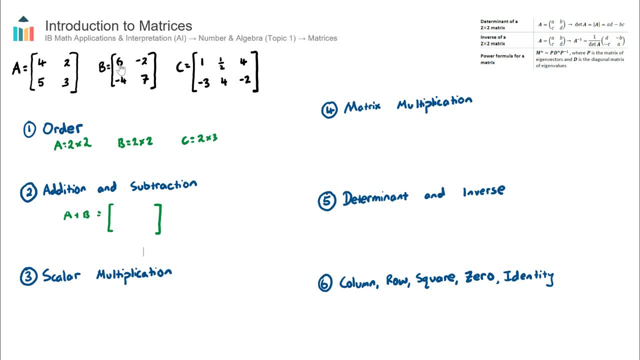 the two top left numbers added to each other, So four plus six. So this top left number here will be 10.. Same for the top right number. that'll be two plus negative two, which is zero. The bottom left number, five plus negative four, is one And finally, three plus seven is 10.. 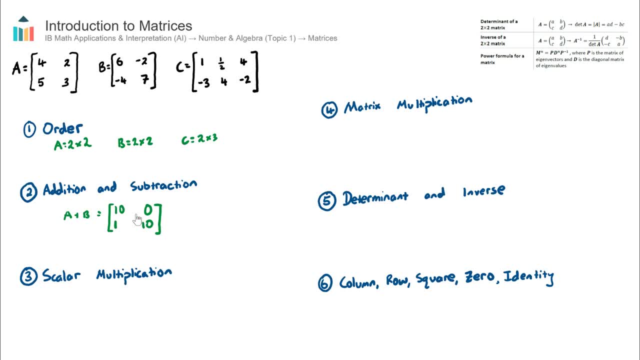 So pretty simple. there, Subtraction works exactly the same, except you'll be subtracting the numbers. So, for example, four take six will be negative, two, and so on and so on. Okay, let's look at scalar multiplication now. This is when we multiply a matrix by a number which we call a scalar rather than. 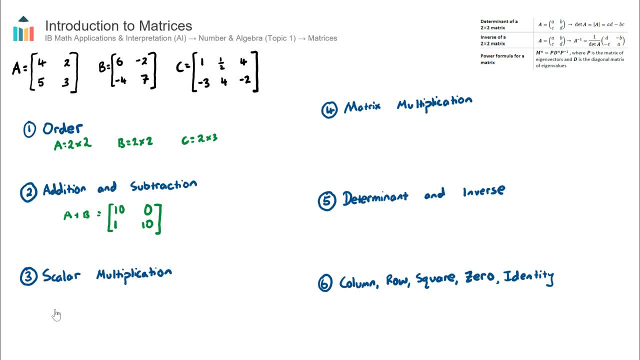 multiplying two matrices together. So, as an example, let's look at three multiplied by matrix A, And we can write that as three outside of the matrix A, which is four, two, five, three, And that will equal. all we need to simply do, there is just multiply this three. 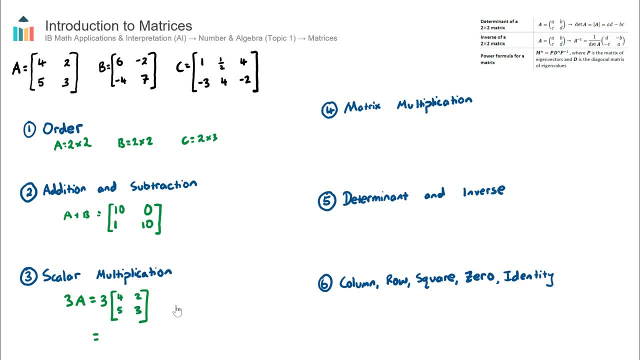 through to every value in the matrix. So this will be: three times four is 12,, three times two is six, three times five is 15, and then three times three is nine. So that's all there is to it there, You. 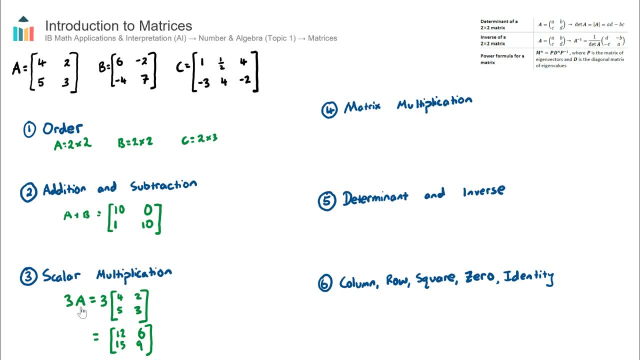 often see fraction scalars as well. So, for example, half A same process. you would just multiply a half or maybe 0.5 through to every value in the matrix. So that's all there is to it there. You would just multiply a half or maybe 0.5 through to every value in the matrix that you're multiplying. 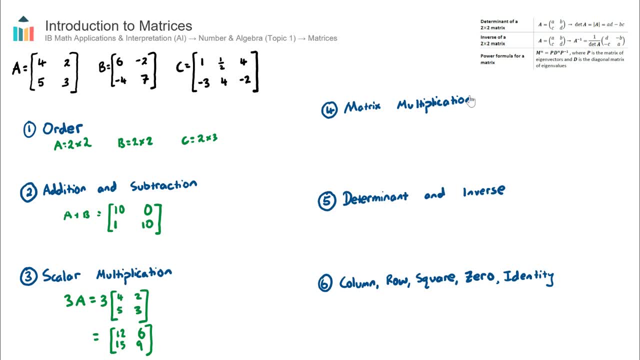 the scalar by, Okay, matrix multiplication. Now this is a little bit trickier. Before we go ahead and multiply two matrices, we need to test whether we can actually multiply them together, And the way that we do that let's consider. I'll just put to the top here. Let's say that we're trying. 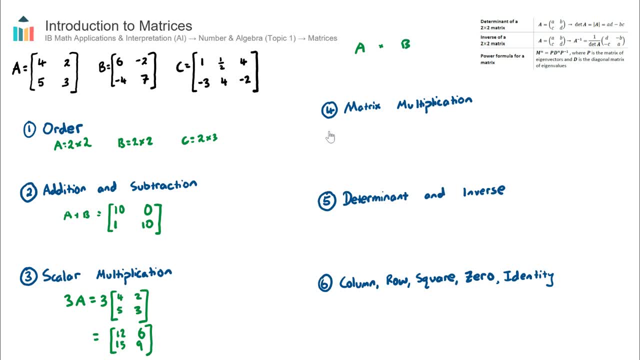 to multiply matrix A by matrix B. Well, underneath these two, I'm going to write the order. So let's say two by two, and the matrix B is also two by two. If I want to multiply these two matrices, the middle numbers here need to be the same. So this is. that is the case in my example here. 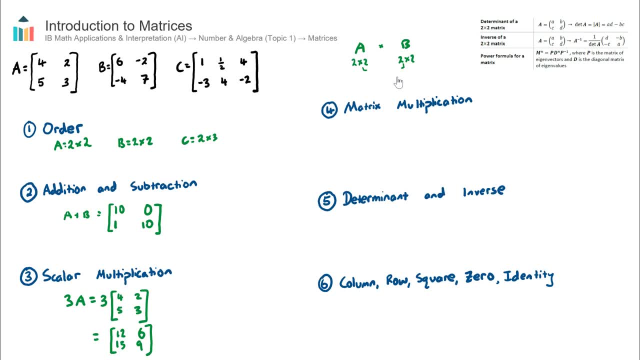 two and two. So therefore I can multiply these two matrices together And the resultant matrix will be the order of the outside numbers. So my result will be a two by two, If I wanted to multiply, say, A by C. so there'll be two by two and a two by three. I can multiply these two. 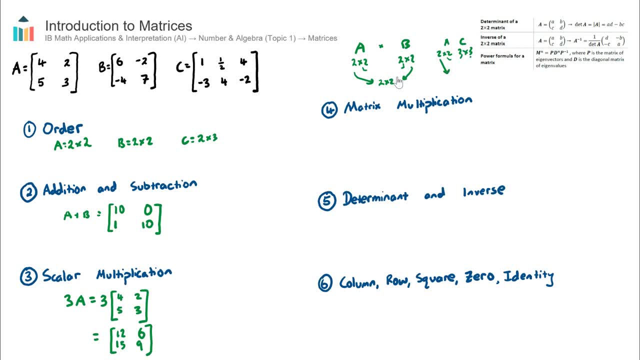 matrices together because the middle two numbers are the same And my result is actually going to be a two by two. So I can multiply these two matrices together because the middle two numbers are two by three. Okay, so let's go ahead and multiply matrix A by matrix B. This does take a. 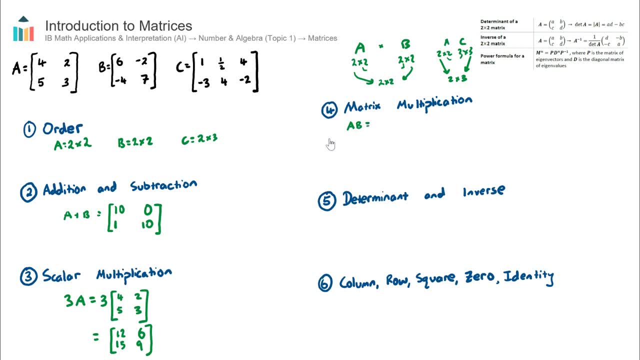 little while. So A times B. I have already tested that I can do this, And I already know that the resultant order will be a two by two What I do here. I'm going to just pause the video and write these matrices. Okay, this takes a little bit of practice, but let's focus on this topless cell. 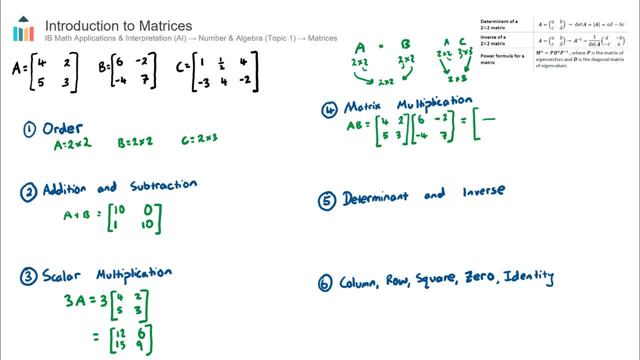 here. The way that I find this number here is I multiply across the row, So across- I'll use a different color Here- across the row and then down the column, So this will become: it'll be four by six plus two. 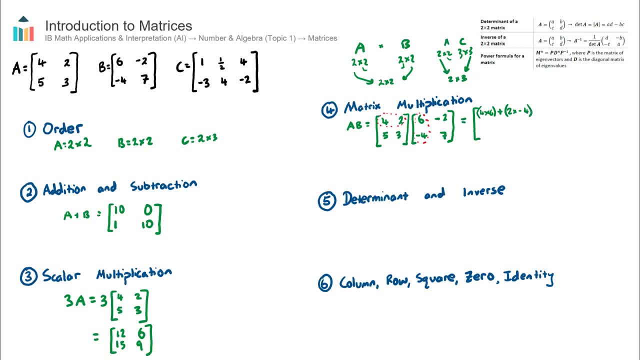 by negative four. Let's now focus on the next number here, the top right. Again I go across- I'll use a different color again- across the row Here, across the row and then down the column. It takes a little bit of practice to get. 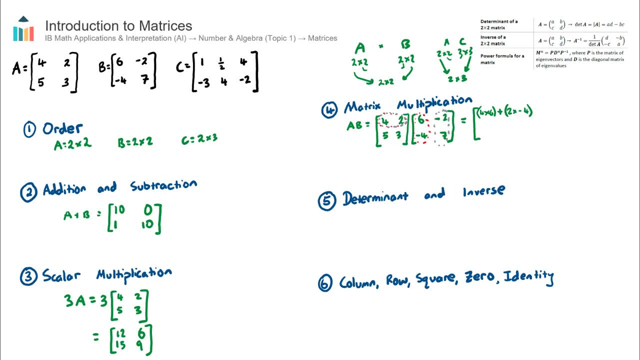 comfortable with this. but after a while you start to get a feel for the pattern. So this one here will be four, by negative two plus two by seven. Okay, I'll just quickly finish off the other two values. This one here will be five. So again, I'm going through this row. now the bottom. 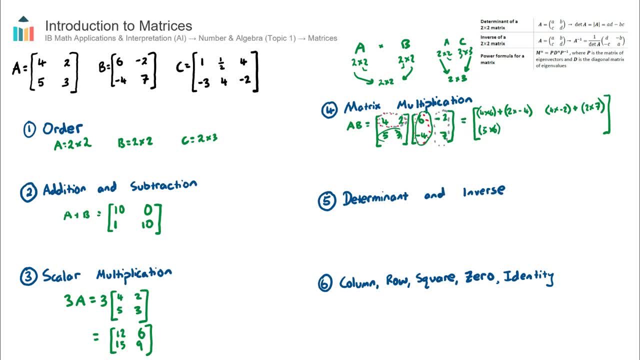 right value will be five by six plus three by negative four And the bottom right value will be five by negative two plus three by seven And that will equal okay. this topless value will be 24. take eight is 16.. Top right value will be negative eight plus 14, which is six. Bottom left value. 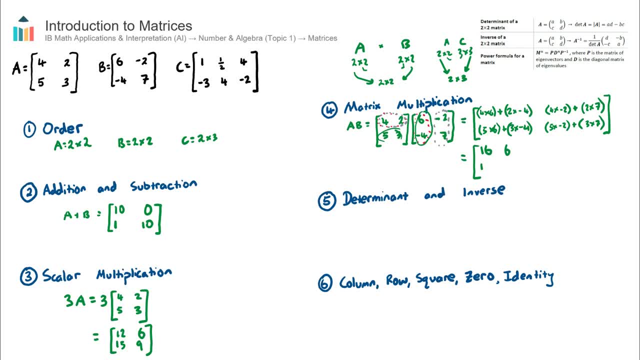 will be 30 take 12, which is 18.. And the bottom right value will be negative: 10 plus 21,, which is 11.. Okay, so there we have it. we have multiplied two, two by two matrices together to get a matrix. 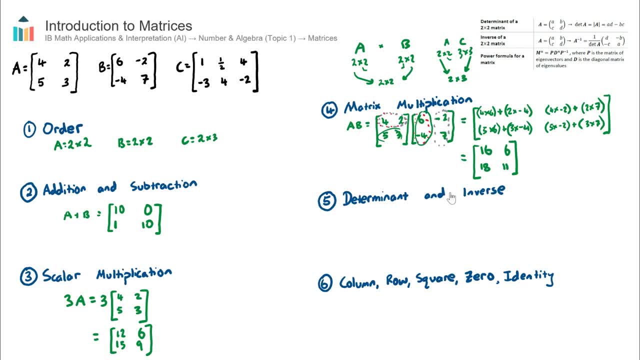 multiplication result. Okay, let's now move on to determinant and inverse. I'm going to focus on matrix A. We actually have formulas. There are three formulas given in the AI formula booklet for matrices. The first two involve the determinants And the second two involve the 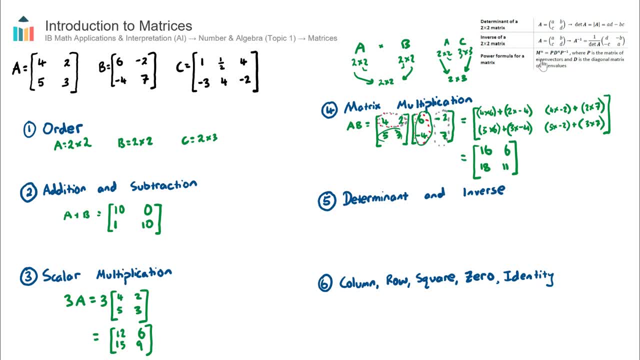 determinants, And the third two involve the determinants And the fourth two involve the determinants And the inverse. And then the third one is around finding the power of a matrix, which we focus on in a video titled matrix powers later on. But let's now find the. 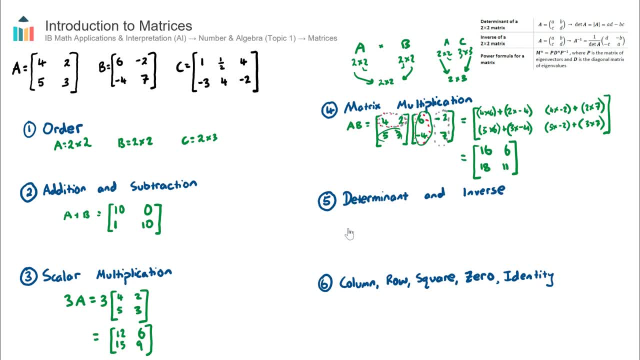 determinant of matrix A And we call that det A determinants of matrix A. And we can also show that in symbol form like this: And that will equal. let's have a look at the formula here. So it's AD, So it's the top left multiply the by the bottom right subtract. 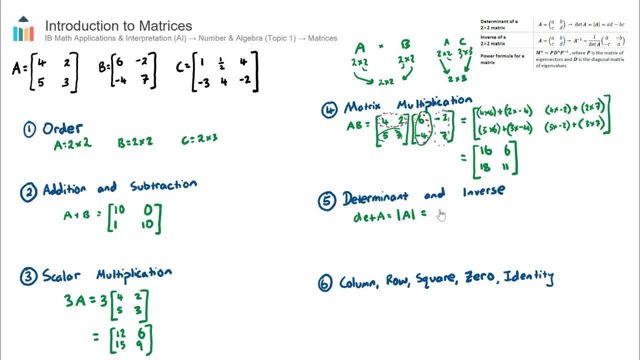 the top right multiply by the bottom left. So in our case here this will be 4 times 3, subtract 2 times 5.. So 4 times 3, subtract 2 times 5. And that is 12 take 10, which is 2.. Okay, so we have just 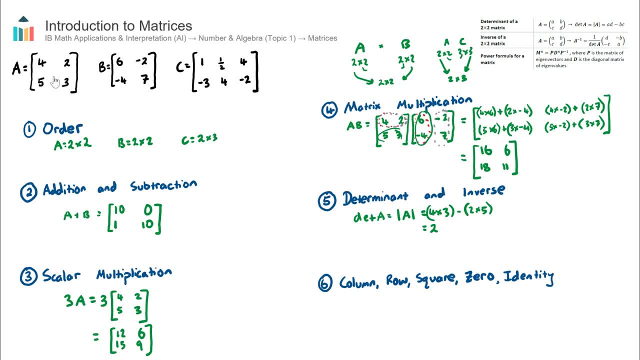 found the determinant of matrix A. Let's now continue on and find the inverse. So the inverse which we denote- as I'll write it, inverse, But we denote that as A, to the power of negative 1. That is equal to. 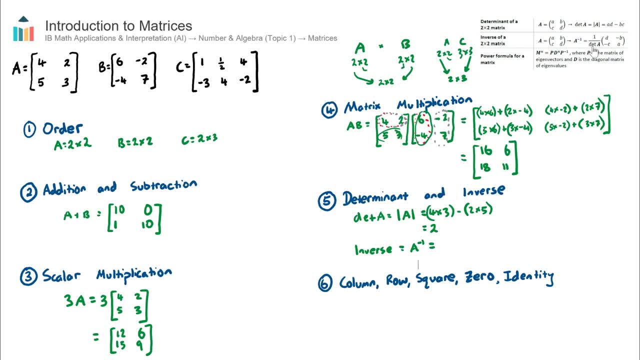 let's have a look at the formula here. It's 1 on the determinant of A, which we just found to be 2.. So it'll be 1 on 2.. And then the result here. it's an interesting result. I won't go through the. 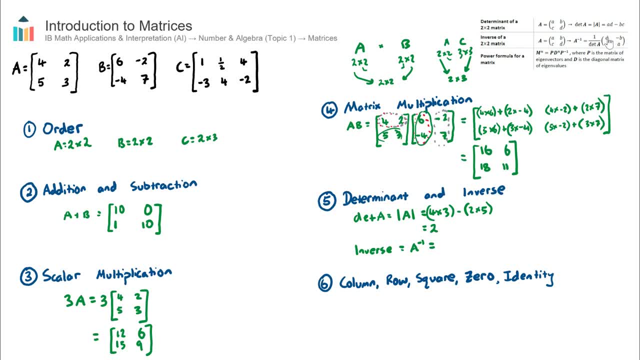 proof of this, because it'll probably take a little bit too long, But in order to just remember it, or you can just refer to your formula booklet, the A and D are swapped, So this top left and bottom right are swapped around And the other two values are the same. So the other two values are: 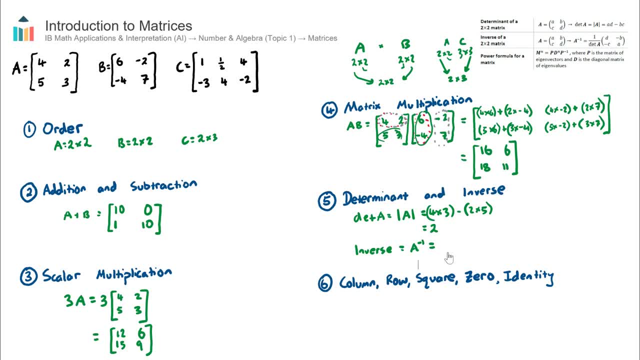 become negatives, So this will become 1 on the determinant of A, which is 1 on 2.. Outside of, let's swap our A and D around, So 4 and 3, that'll become 3 and 4. And our other values stay in the. 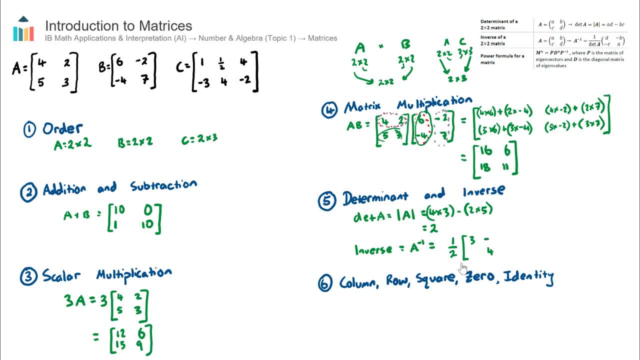 same position, but they turn negative. So negative 2 and negative 5.. Now we can multiply this scalar of a half through our matrix, And we covered that back in point 3.. So let's go ahead and do that. I'll just go across the page here. 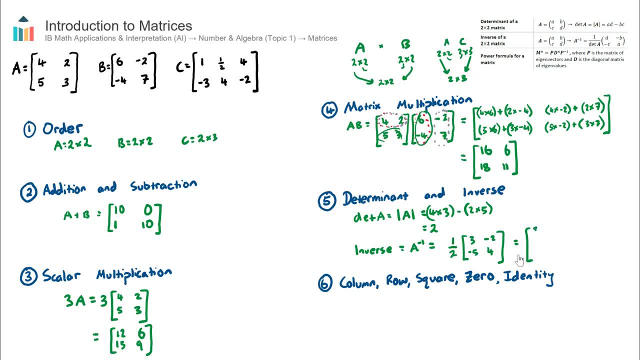 Multiply our scalar of a half through. This will be 3 on 2.. Negative 2 multiplied by a half will just be negative 1.. Negative 5 on 2, I can just write as negative 5 on 2.. And then 4, a half times. 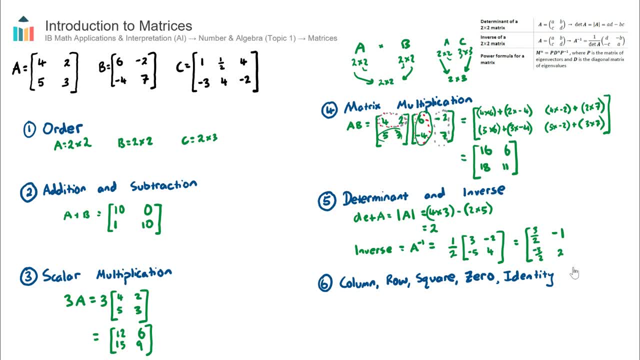 4 will just be 2.. So there we have it. We have just found the inverse of our matrix A. Okay, I'd just like to finish by going through some terminology with matrices that you'll see. It's important to sort of understand what these words mean. So the first one here: 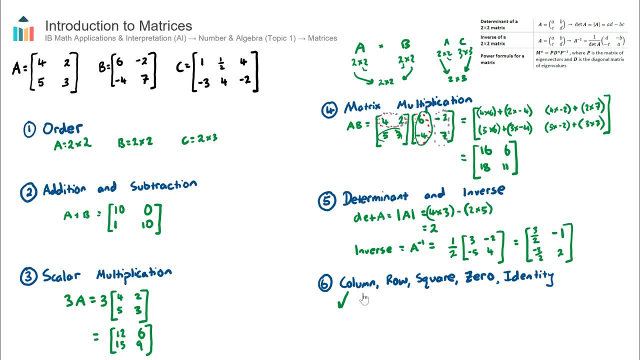 what is a column matrix? A column matrix is a matrix that has one column and many rows. So an example of this would be: so one column, many rows. It might be say 2,, 5,, 7.. That has one. 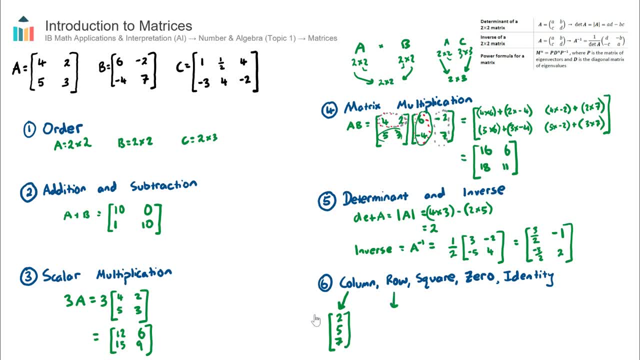 column and three rows And, as you could probably predict, a row matrix will have one row and many columns, So that might be, say, 3,, 8,, 12.. One row, many columns, So in this case, three columns. 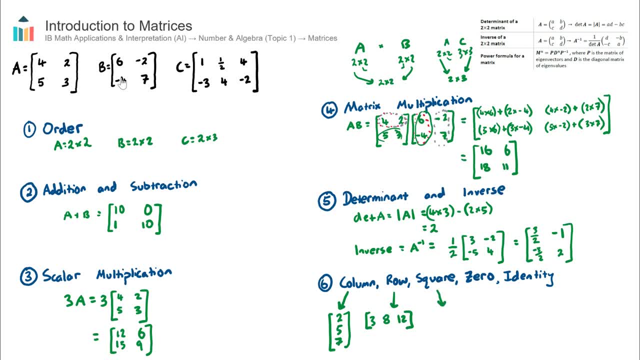 Now we have two examples of square matrices up above here. So A and B are square matrices, That's when the order is the same. So, for example, 2 by 2, or 3 by 3, or 4 by 4,, etc. And as you can kind. 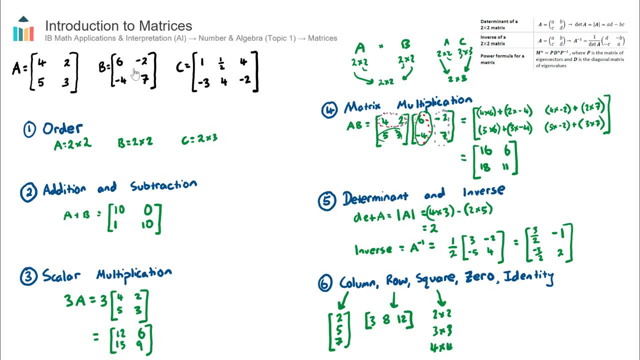 of tell, they actually result in a square as opposed to a rectangle, A zero matrix. that is, when all the values in the matrix are zero. So, as an example of a 2 by 2 square zero matrix, that would be 0, 0, 0, 0.. 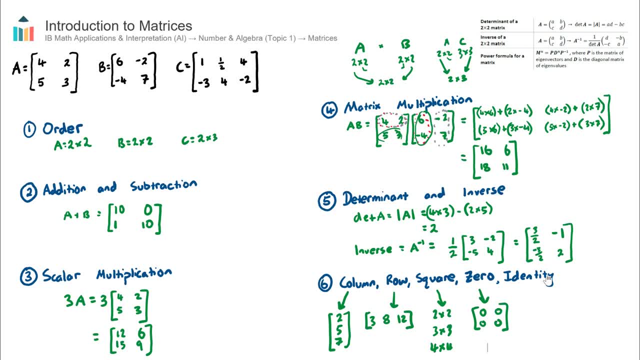 And finally, the identity matrix- very important, this one here. We're actually going to deal with this in the next video- involving solving simultaneous equations. That kind of acts like the digit 1 in matrices: land, And what that looks like is a square matrix where the diagonal 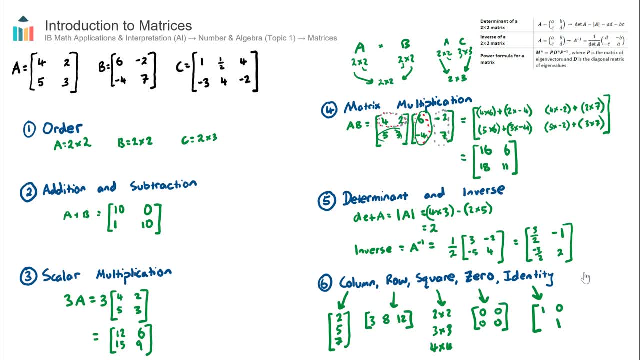 top left to bottom right are ones and every other value is a zero. So that's the example there of a 2 by 2 identity matrix, and we call that I A. 3 by 3 would be 1, 1,. 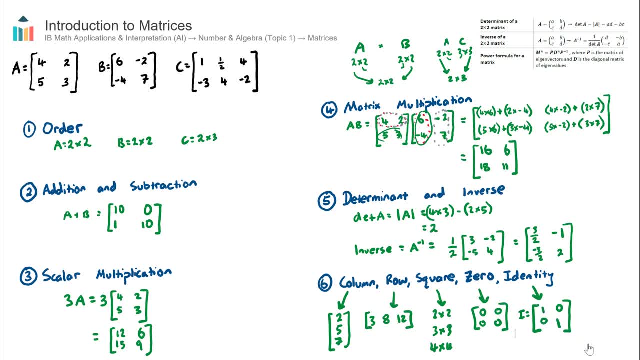 1 going down the diagonal top left to bottom right and all the other values are zero. Okay, that concludes our introductory video to matrices. 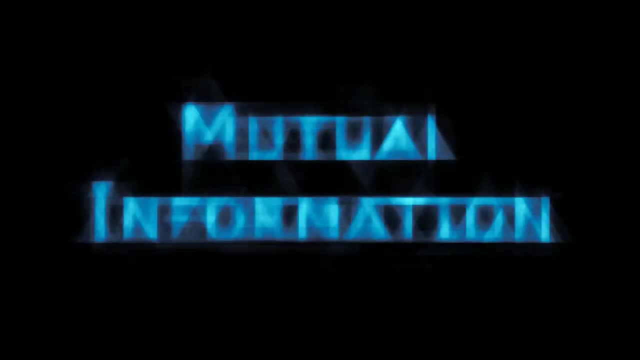 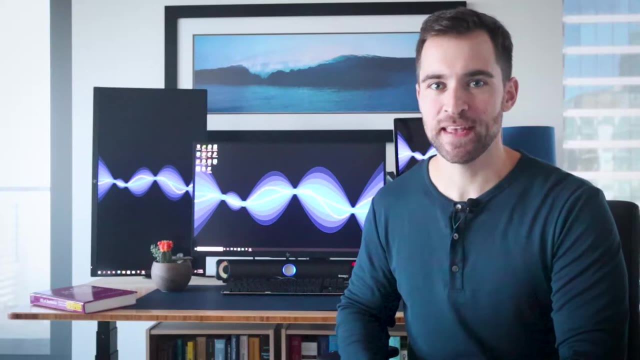 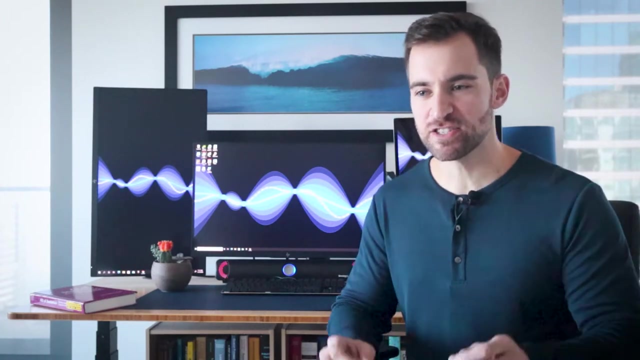 Welcome to Mutual Information. my name is DJ. In this video I'm going to show you what I think is the best approach to learning about probability distributions. I'll start with an analogy. Let's say you had a full minute to memorize this mess. After that minute, 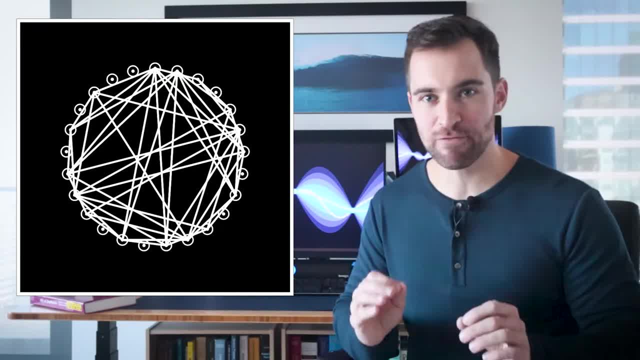 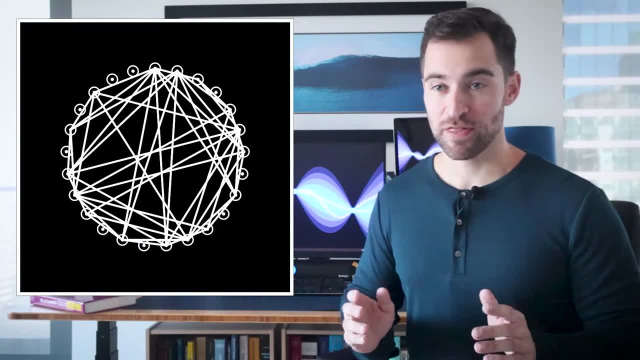 you have to redraw it from memory perfectly, Every edge, every node, no mistakes. You think you can do it. Well, if you have a normal human brain like me, then no, there are just too many details to get wrong. But what if I were to tell you about the pattern behind? 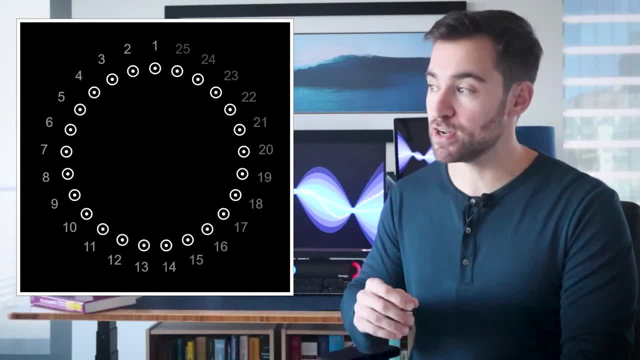 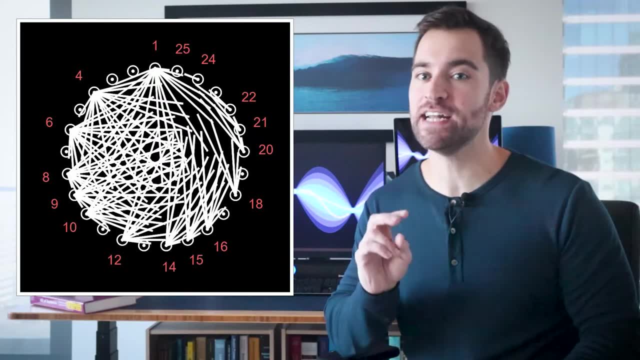 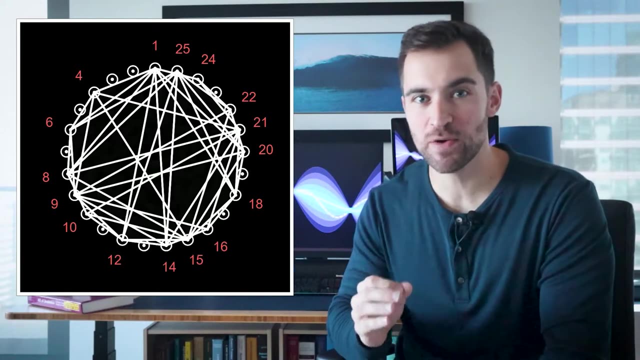 this complexity, That is, there are 25 nodes which can be numbered like this, and you should consider only nodes that are not prime. Then draw an edge between any two of them, but only if their difference is prime. Now I'll ask again: could you redraw this pattern, knowing? 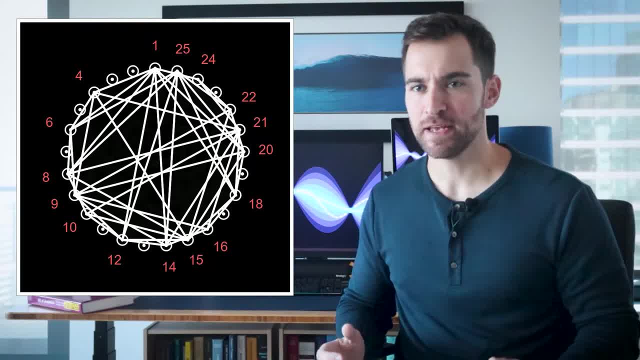 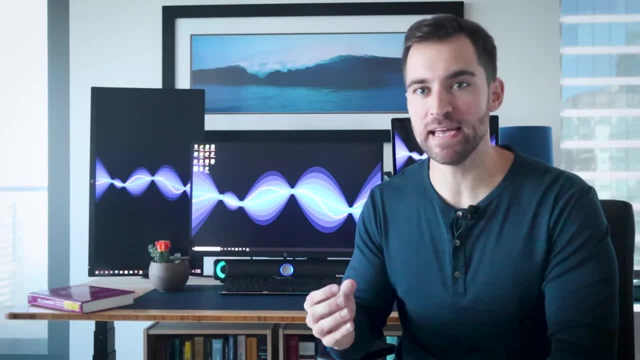 this fact. I mean, yeah, almost certainly It might be tedious and annoying, so please don't do it, But yes, it could easily be done. all from memory. The lesson here is: if you want to hold something big and complicated in your head, it's best.